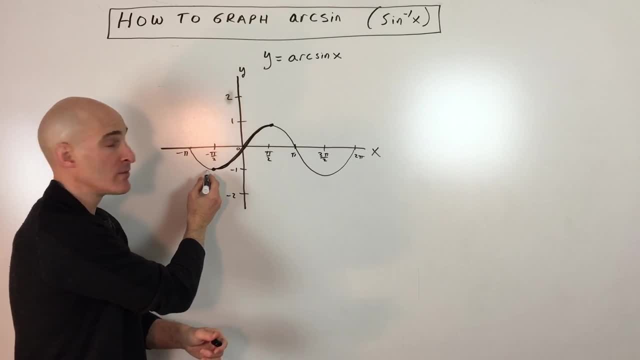 three key points here. Let's look at this point here: negative pi over 2, comma, negative 1.. And what we're going to do here is we're just going to write this out, But what I'm going to do is I'm going to switch the x and the y coordinates. So if we do that, this is going to be negative 1, negative pi over 2.. Now, remember, pi is 3.14 approximately. divided by 2 is about 1.57.. So this point is really going to be negative 1, negative 1.57.. Okay, so if we graph this, 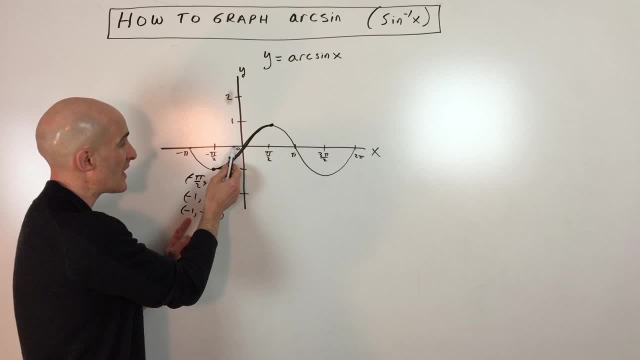 negative pi over 2, this is like negative 1.57.. So we're negative. 1 is going to be right about there. okay, about two thirds of the way, And then we're gonna go down negative 1.57, it's going to be right. 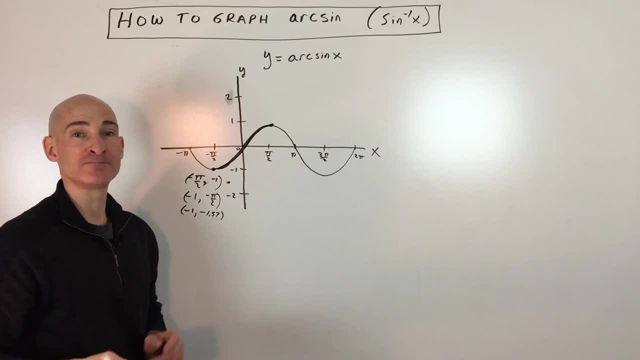 about there. Okay, so you're with me so far. Now the point here where it goes to the origin, that, of course, is 0, 0.. And when you interchange the x and the y coordinates there, it's just the same. 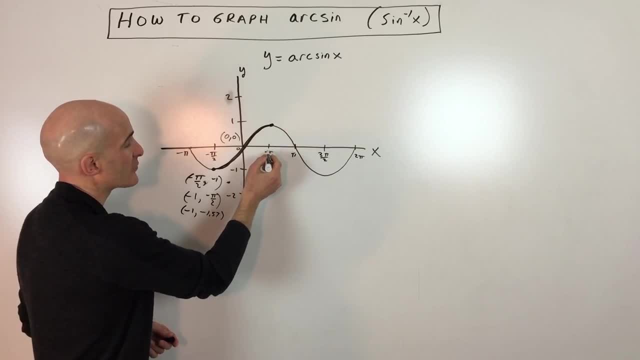 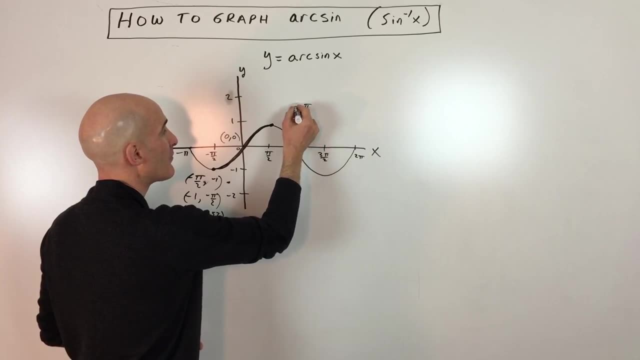 exact point. Okay, so we're going to be right there. And then this other point: pi over 2 comma 1, let's mark that one down. pi over 2 comma 1, if we switch the x and the y, we get 1 comma pi over 2.. And again, pi over 2,. remember is about. 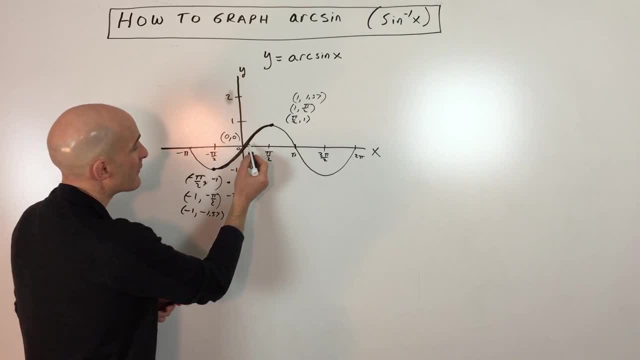 1.57.. Okay, so what we're going to do is we're going to graph that point. So 1 is going to be right about here. Okay, this is 1.57.. So this is about two thirds of the way, Okay, and then we're. 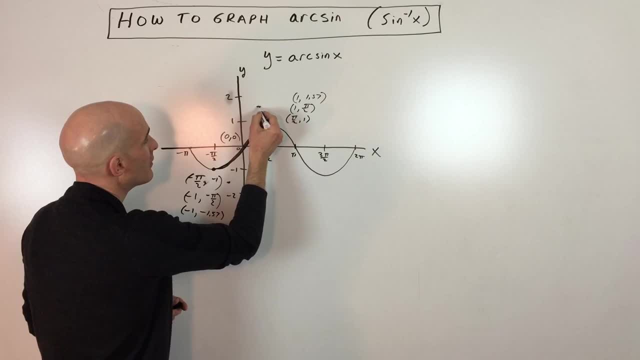 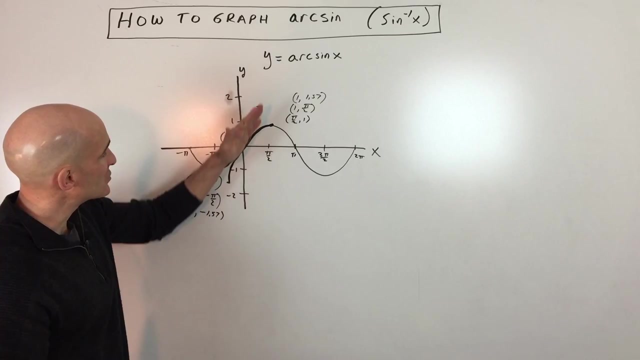 going to go up 1.57, which is right about there. Okay, now, when we graph this, the graph is going to look like, let's see, like this. Now, one thing that you'll notice when you graph the inverse function: it's going to be a reflection. 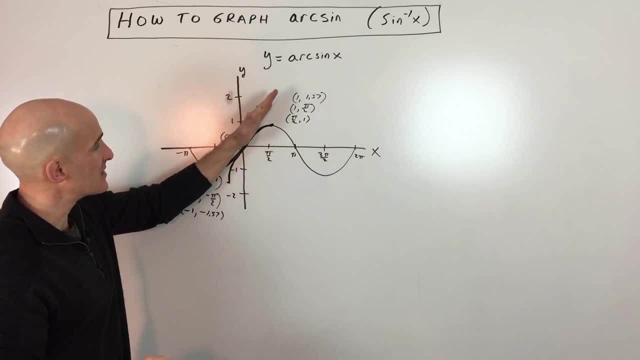 over the line. y equals x, So it's a line that has a slope of one. It's like a 45 degree line And it's going to be a reflection, okay, over that, over that line. So that's all you have to do If 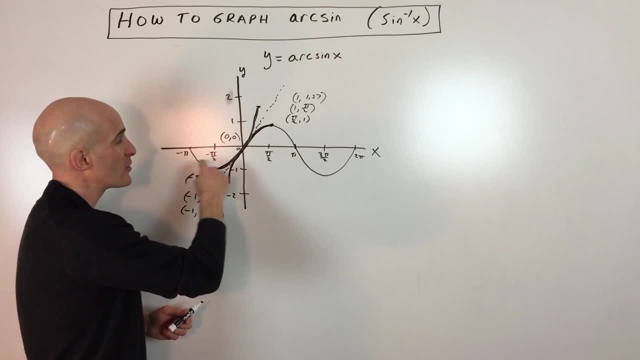 you forget how to graph the arc sine or the sine inverse function, go ahead and graph the original graph, restrict the domain from negative pi over 2 to positive pi over 2, and then switch the x and the y coordinates on these three key points And that'll be a quick way to graph the inverse function.